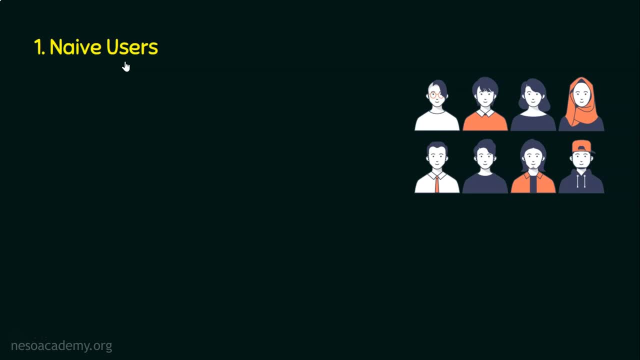 whoever wants to book a train ticket. they should know the technology. No, So they should know only how to use the system. They may not be needed to know the working or the technical specifications or the technical details about the system. So basically, naive users are unsophisticated users. 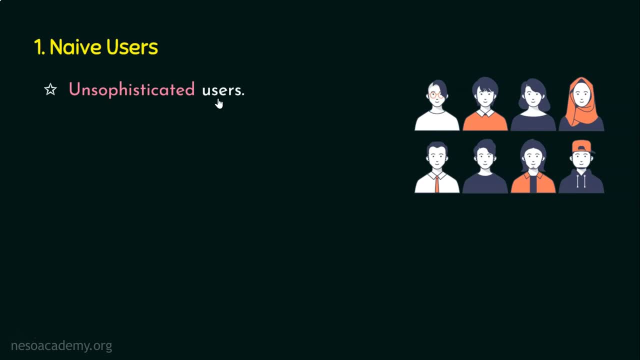 where they lack the technical knowledge. In this subject, naive users are referred as unsophisticated users and they lack database knowledge And what they are required to know. They are required to know how to use the system right, Because already the application programs are well written and they 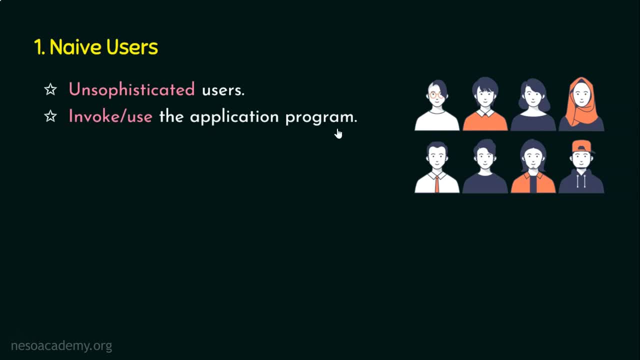 are going to just invoke or use the already written application programs. Say, for example, if you're going to an ATM machine to withdraw money, you should know how to operate the system. That's it, Because how to withdraw the money, everything is predefined using the application programs. 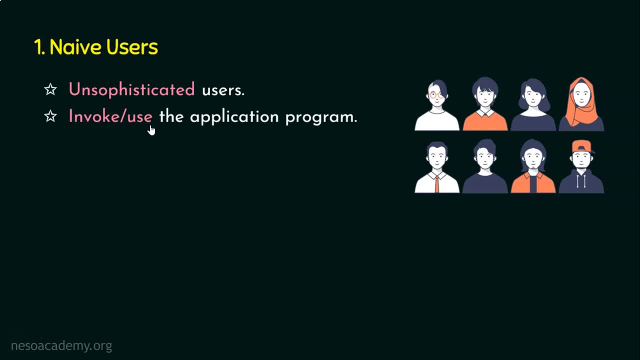 And these naive users are going to invoke or use the application programs that was already written. I'll give you some examples: Clerk tellers in the bank, because they know how to access the system And when some customer comes and asks for certain details. 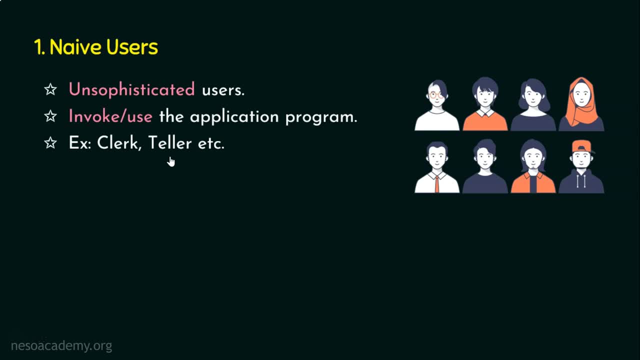 they will be able to provide assistance to the customers by giving the right information, by accessing the data from the database, But please be noted that they are not going to supply SQL queries in order to fetch the data. They know how to use the system, How easily we can access the. 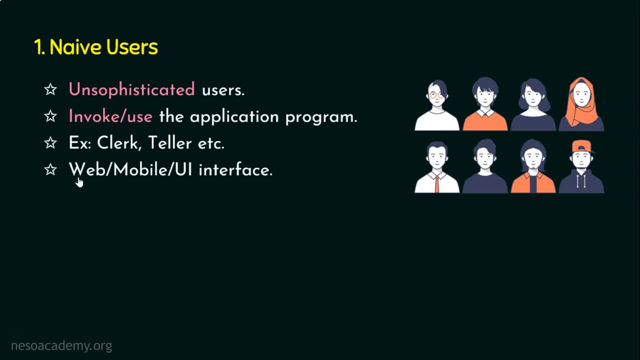 database system, Because we are in a contemporary world where we have multiple webpages, web interfaces, mobile interfaces, user interfaces are defined. Say, if you want to book a movie ticket, are you preferring to go to the movie theater to book a ticket? No, we are not preferring. 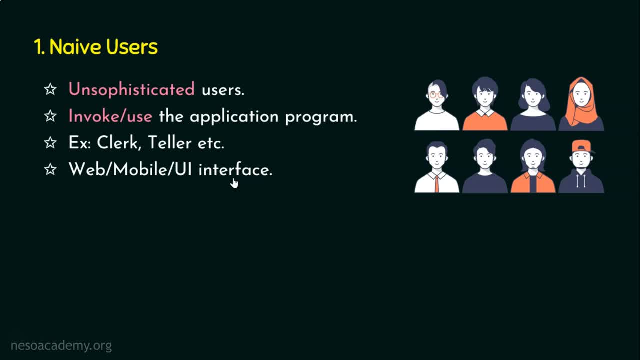 that nowadays, From my mobile phone or from my laptop or from my desktop, I can easily book a movie ticket or a train ticket or a flight ticket. Even I can purchase goods online. So users are expected to know how to use the system And, as mentioned, we also have some desktop applications. 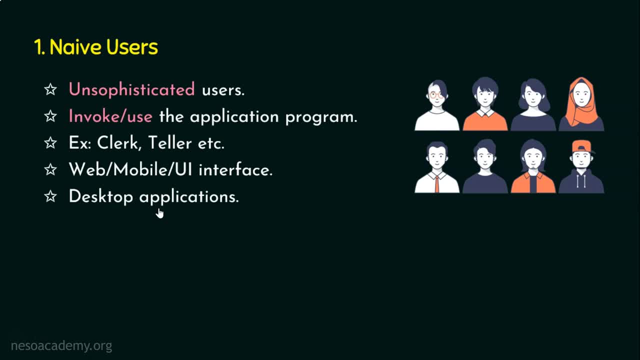 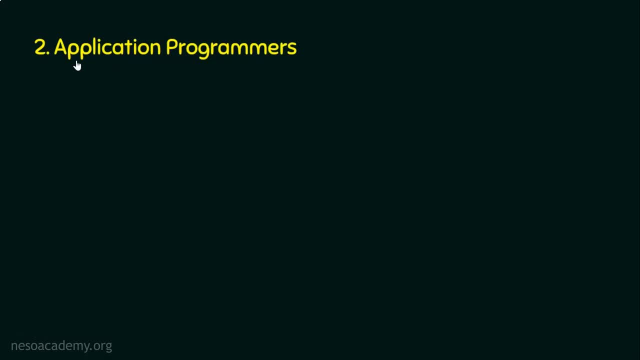 and we should know how to use the system. That is the only requirement for the users. So we are done with the first type of users, the Naive users. Let's now move on to the second type of users, the Application Programmers. 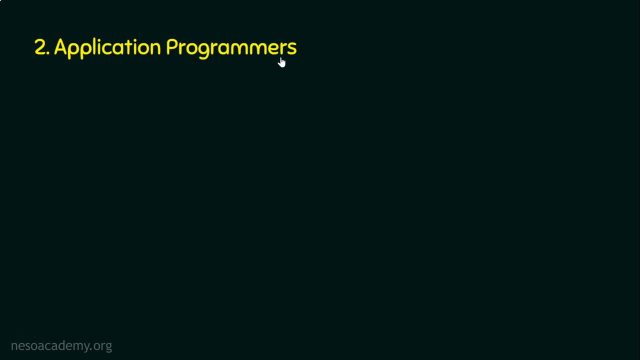 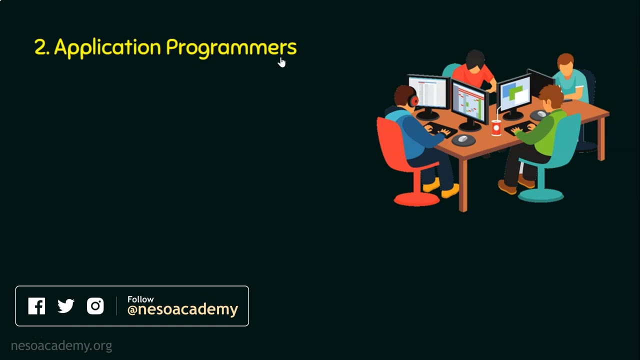 We know Naive users are going to use or invoke the application programs that was already written. Who has written those application programs? The application programmers, the software developers, right? So these software developers or application programmers are computer professionals and they are specialized in development of the software. In other words, 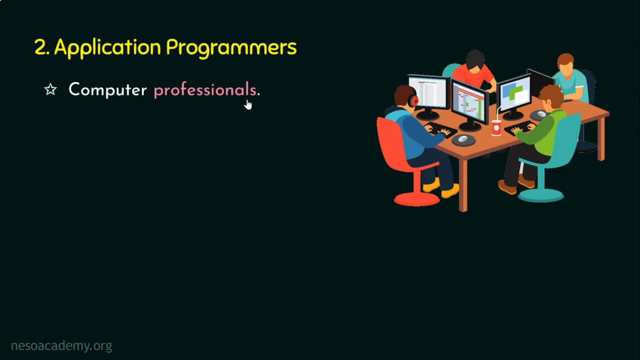 we can also say that they know some programming languages, how to write a program, how to create a software, how to write an application as well. When they know how to develop an application, they obviously use some application development tools and other tools and technologies that are: 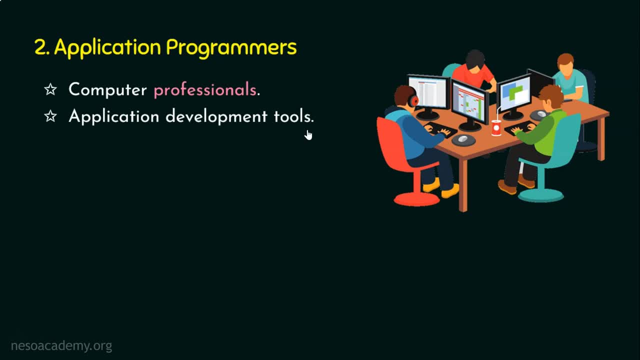 required to develop an application And obviously, what's their main job Is to develop the user interfaces that are really user-friendly and easy to access, because they are going to develop the application programs which are not going to be used by other software professionals. 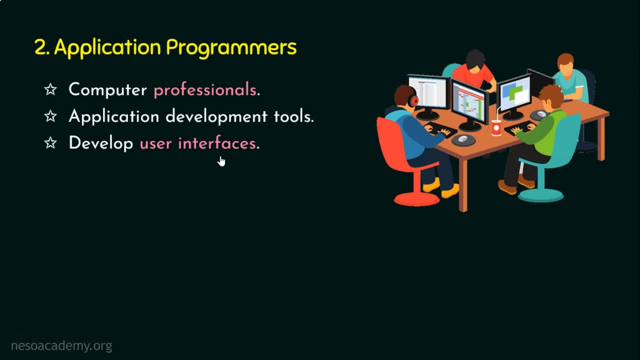 The applications that they develop are going to be actually used by Naive users also. So in that case, the system or the application they create, in other words, the user interfaces they create- it should be user-friendly, And obviously the application developers use rapid application. 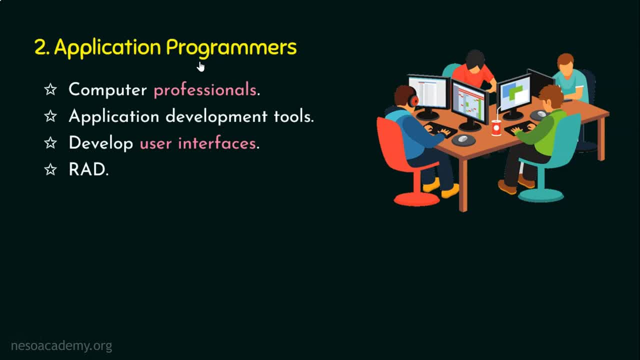 development tools for developing the application programs And, obviously, what these application programmers are going to develop: Applications or web or mobile interfaces, To be precise, they are going to develop user interfaces that are really user-friendly. So we are done with the second type of users, the application programmers. 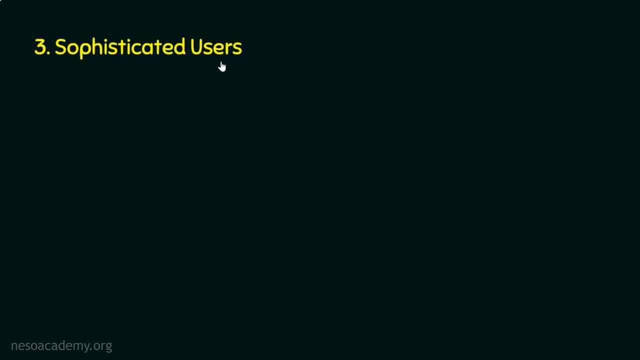 Let's now move on to the third type of users, the sophisticated users. We know Naive users are unsophisticated users, but now we are talking about sophisticated users, So obviously they know the nook and corners of the system and they also know how to interact with the system. These sophisticated 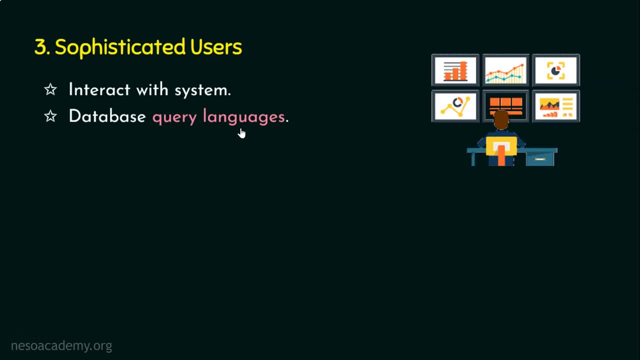 users. they use the database query languages because they know how to interact with the system. Let's take the database Administrator as an example. he is a sophisticated user How He knows how to write queries in order to fetch the information from the database. So sophisticated users. example- database administrator. 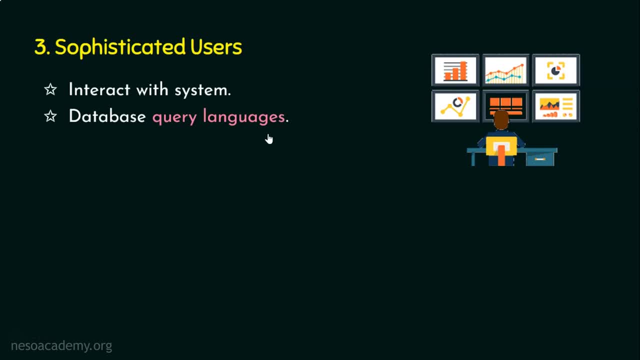 knows how to use the database query languages And also they know how to use data analysis software, because they are directly interacting with the database. database contains data and not only they are going to use the queries for just fetching the data or storing the data, they also. 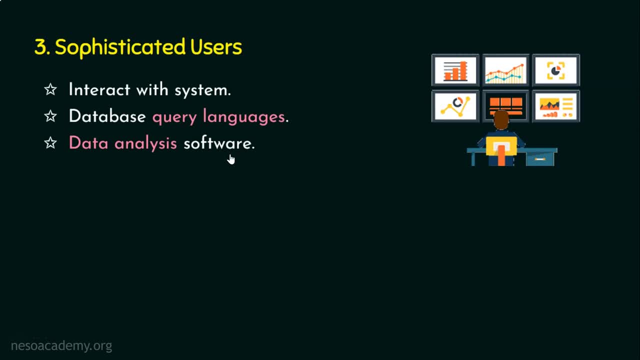 know how to use some data analysis software in order to do the analysis. As already mentioned in the first lecture of the subject, today there is a need for data analyst and business analyst in the job market, So these users will be able to know how to use some data analysis software. So we are done. 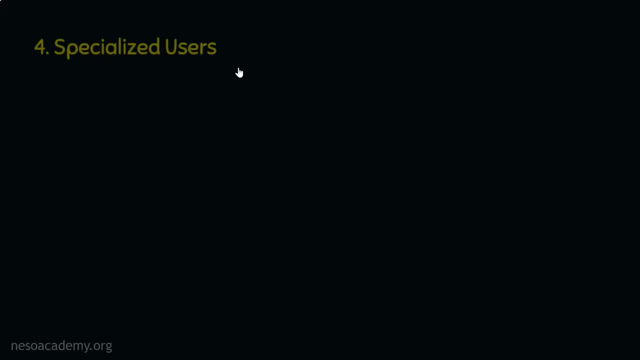 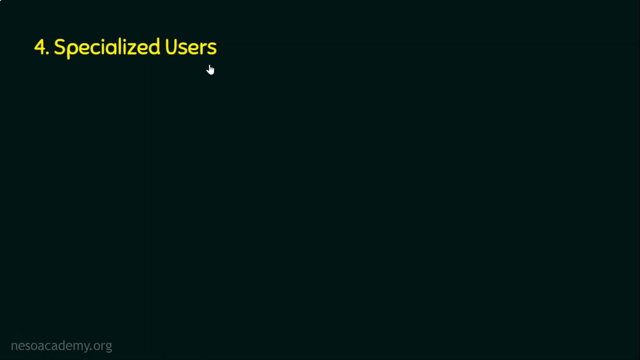 with the third type of users, the sophisticated users. Let's now move on to the fourth type of user, the specialized users. The name itself says that they have additional skill sets. In other words, they have some specialized skills. What type of users they are The specialized users are: These users are specialized to use some. 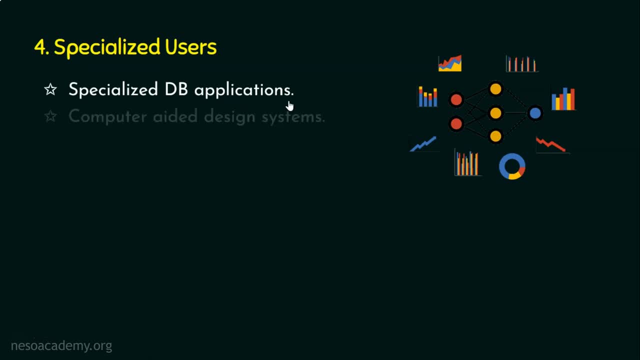 database applications, Not only simple database access. they also have some specialized database applications. Say, for example, they will be proficient with computer-aided design systems. We can see a lot of innovations in the artificial intelligence area, So specialized users will have. 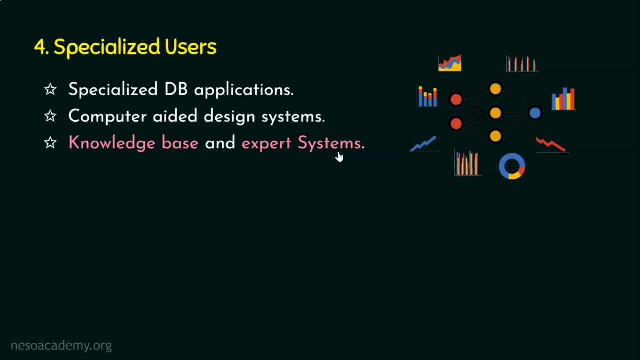 knowledge about the knowledge base and expert systems. And not only this. the specialized users deal with simple databases. They will also be dealing with the multimedia databases as well. They know how to create a database, how to access the database when it deals with the multimedia 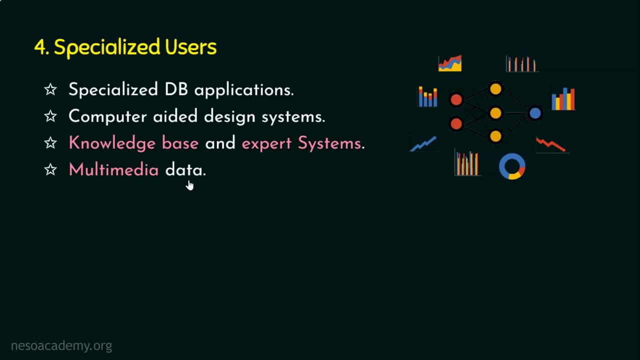 data. What's a multimedia data? It's not simply the text data, It is the audio data, video data, text, animation, graphics, images, whatsoever. And these specialized users are working for the projects that can be deployed in the current and even in the next generation. So we are done with 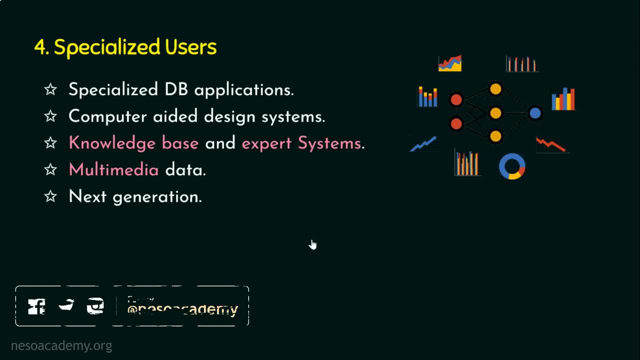 the specialized users. also In this presentation we have seen four different types of users of database: Number one, the Naive users. Number two, application programmers. Number three, sophisticated users And number four, specialized users. And we have a very important user in the database. Who is that, The database? 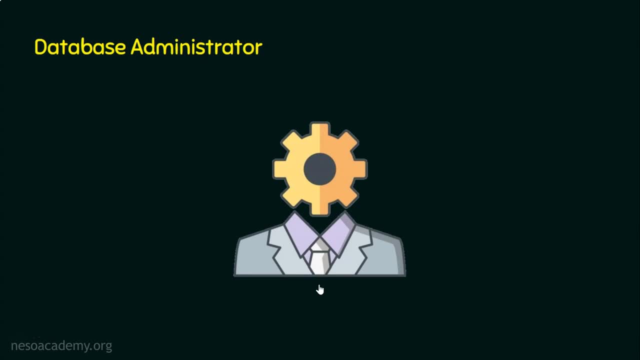 administrator. In the next presentation we will see elaborately about the database administrator and the roles and responsibilities of a database administrator. Please be noted that it's a high privilege to be a database administrator. So let's get started And that's it, guys. I hope you guys enjoyed this presentation And thank you for watching.